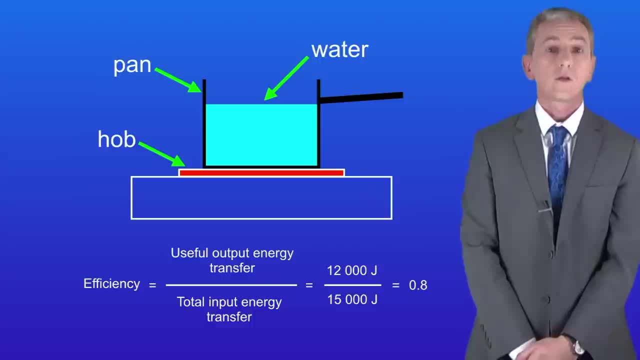 Now there are a couple of points about this that you need to learn. Firstly, we've calculated efficiency as a decimal, and that's fine. You're expected to do that in your exam. However, we can also calculate efficiency as a percentage, and to do that 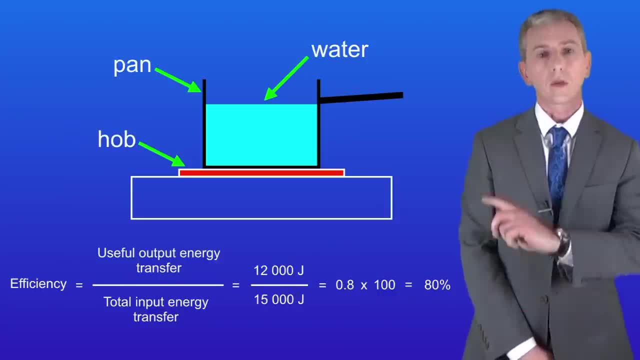 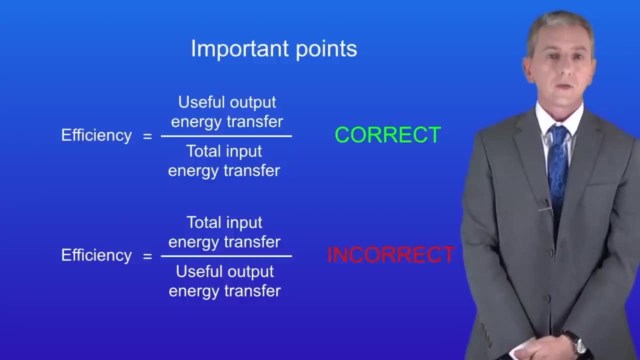 we multiply our decimal value by 100 like this: Now you could be asked to do that in your exam as well. The second important point is that most students who struggle with calculating efficiency write the calculation upside down like this: Now you can tell if you've done this, because you'll. 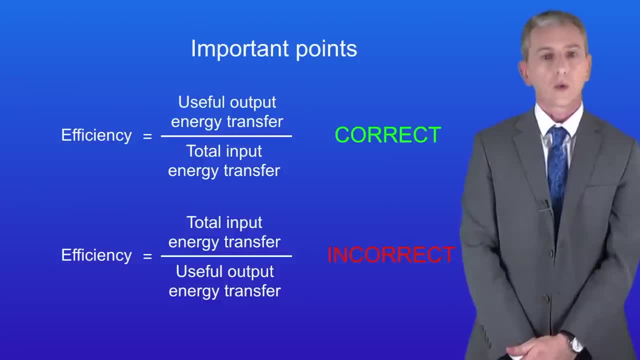 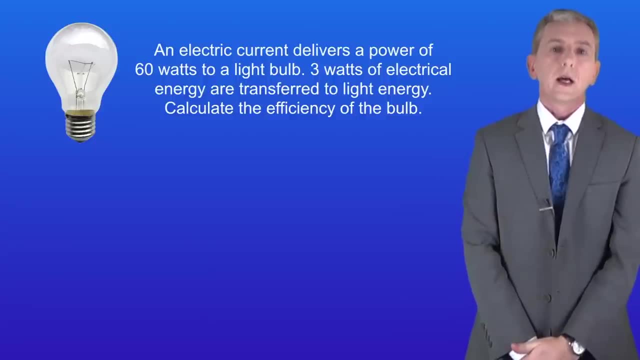 get an efficiency value of greater than one or greater than 100%, And that's just not possible. Here's a question for you to try. An electric current delivers a power of 60 watts to a light bulb. Three watts of electrical energy are transferred to light energy. Calculate the. 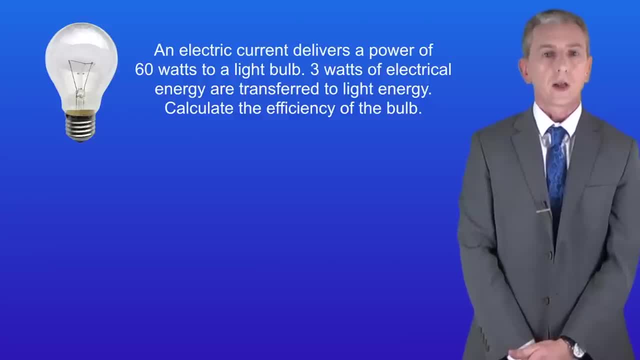 efficiency of the bulb. Okay, pause the video now and try this yourself. So here's the equation that we're going to use. Efficiency equals the useful output, energy transfer. The efficiency is just an equal number. The efficiency of the electrical current is an equal number. We can also calculate. 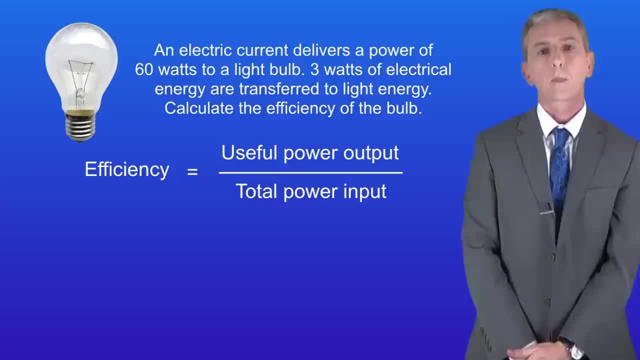 power output divided by the total power input, The useful power output is 3 watts and the total power input is 60 watts. Putting these numbers into the calculation gives us an efficiency of 0.05 or 5%. So, as you can see, 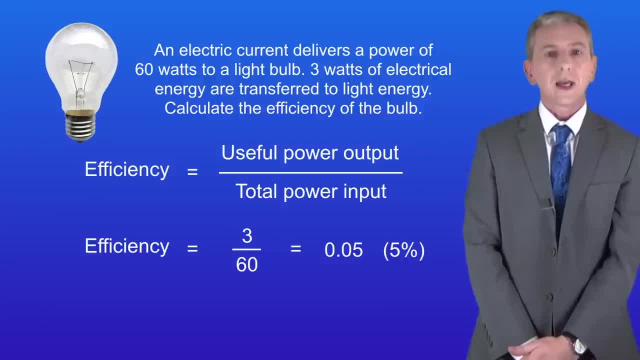 these bulbs are not efficient at all. In fact, most of the electrical energy that these bulbs receive is transferred into thermal energy, which is simply wasted. LED bulbs such as the ones we saw before are much more efficient, as a much greater percentage of energy is transferred to light and much less to 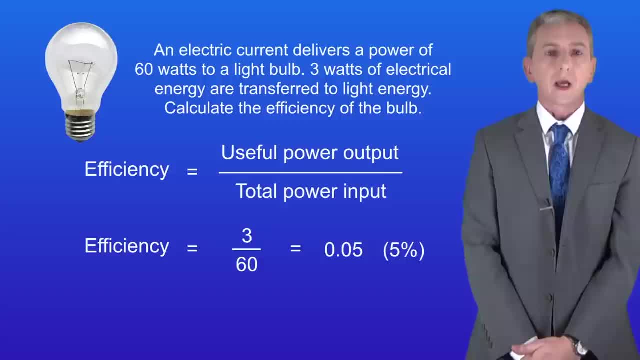 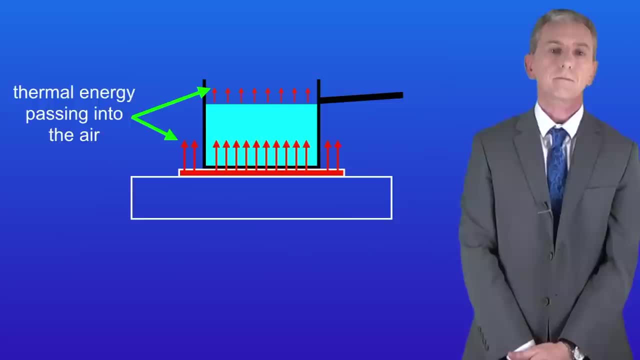 thermal energy. Now in the exam, you could be asked how we can increase the efficiency of an energy transfer. So we're going to go back to the pan of hot water that we saw before. Now, as we saw, this method of energy transfer wasn't. 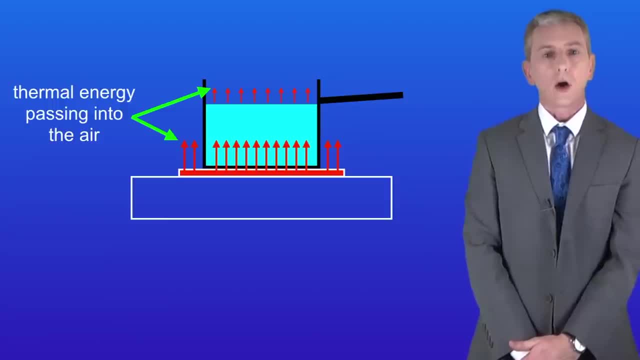 very efficient. We want thermal energy to pass from the hob into the water. However, a lot of the thermal energy is wasted. We've got thermal energy passing into the air around the edges of the hob that are not in contact with the pan. We've also got thermal energy passing into the